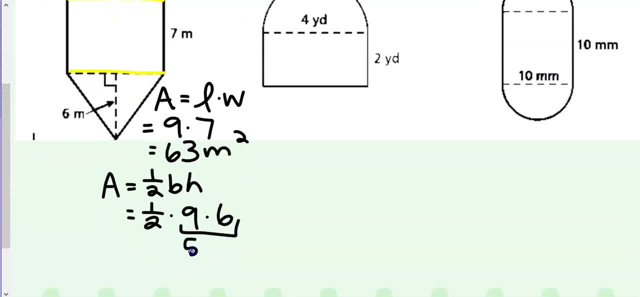 So then, we simply multiply 9 times 6,, which is 54, and we take half of that, which is going to give us 78 square meters. We then take our two areas of our shapes and add them together. 63 plus 28 is going to give me 91 meters squared total for our area of that composite figure. 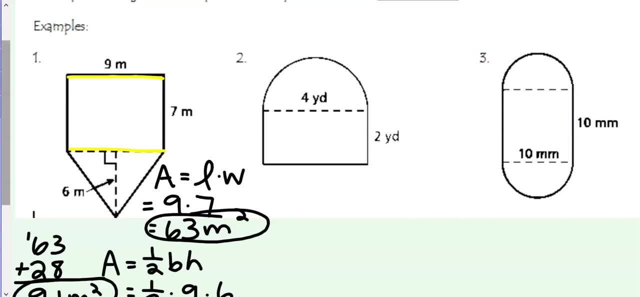 For our next shape, we have a semicircle and a rectangle. So again, the rectangle is going to be area equals length times width, where our length is 4 and our width is 2.. So the area of the rectangle is 8 square yards. 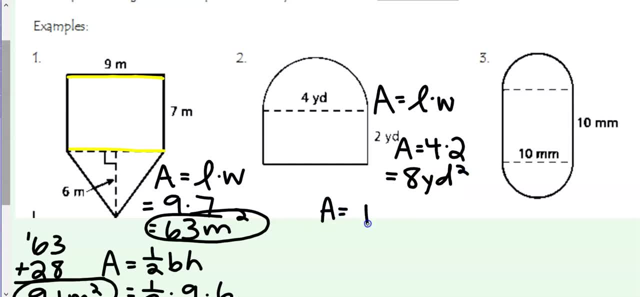 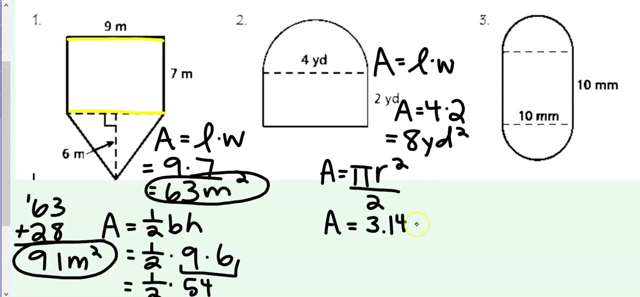 All right, the formula of a circle is: area equals pi r squared. but since we have a semicircle, we have to divide that by 2.. So pi is always 3.14.. Our radius- remember radius- only goes halfway through the circle, which means our radius is 2 because it's half of 4.. 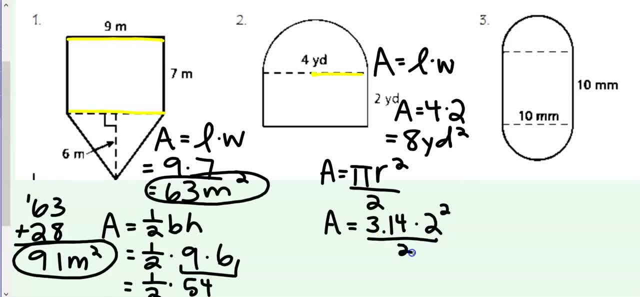 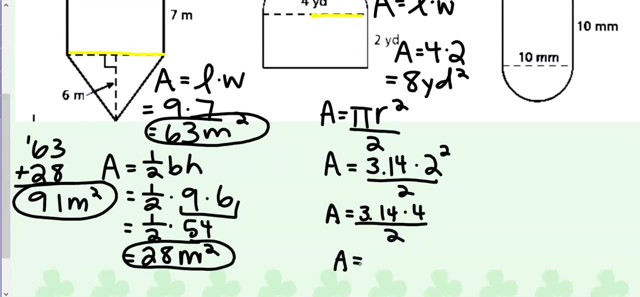 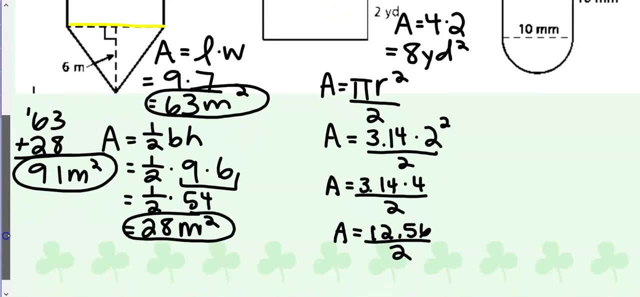 And then we want to square that number. At the end we will divide by 2.. So 2 squared is 4.. Next I want to multiply 3.14 times 4,, which gives me 12.56.. And finally, I want to divide that by 2,. 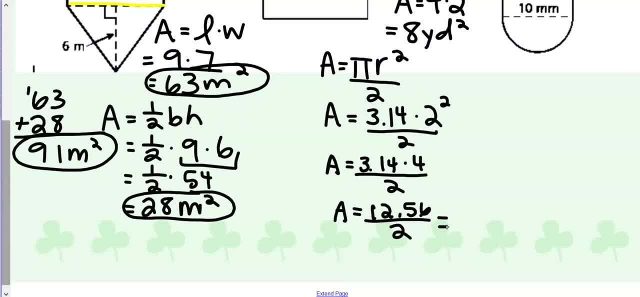 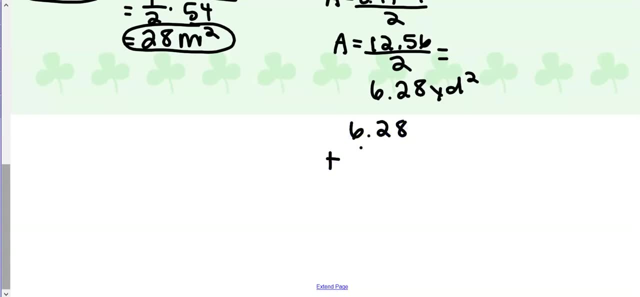 which gives me 6.28 square yards. So to get a final answer for our semicircle that's 6.28 square yards Again, we have to add those two numbers together. So I'm going to take 6.28 plus 8, and that will give me 14.28 square yards. 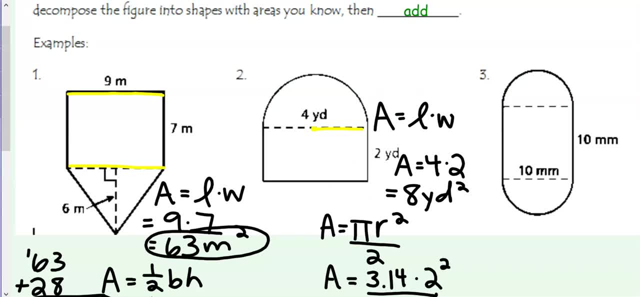 for our entire composite figure. Lastly, we have a square and a rectangle And a semicircle, So we have two semicircles. If I look at these semicircles and took away the square in the middle, it would make a full circle. 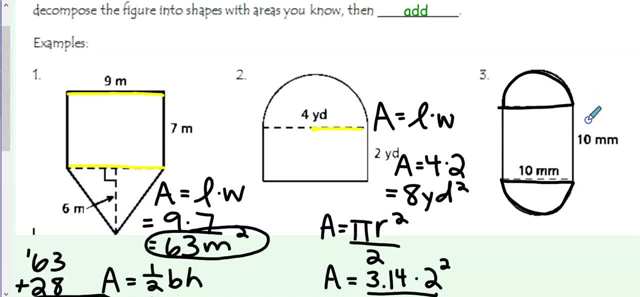 So we don't need to divide by 2 on this one. So first, with our square area equals length times width, which would be 10 times 10 to give me 100 millimeters squared. Then I need to do the circle.